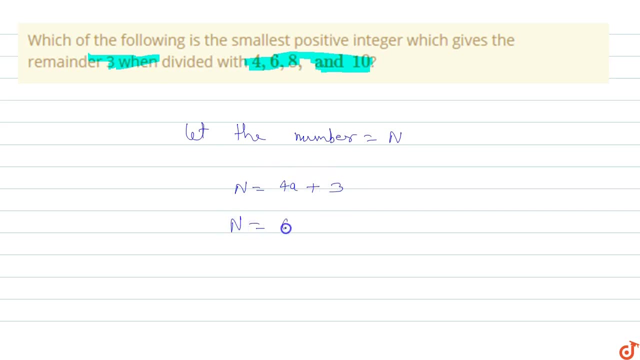 remainder is 3.. This number, n, is divided by 6.. So, and remainder is also 3.. When n is divided by 8, so remainder is 3.. And this n is divided by 10, then remainder is also 3.. So here we can say that n minus 3 equals to 4a and n minus 3 equals to 6b. A, B, C. 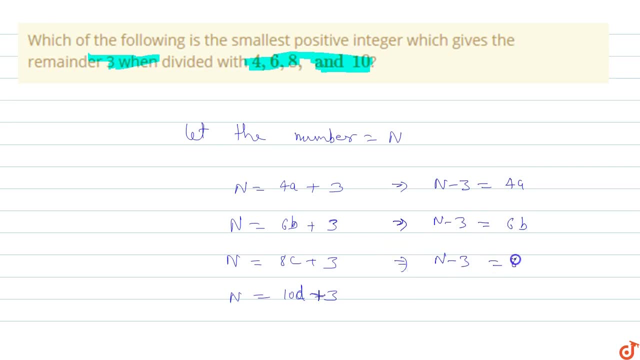 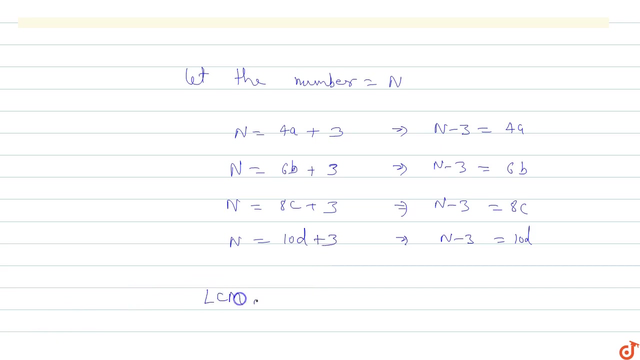 are questioned. So n minus 3 equals to 8c and n minus 3 equals to 10d. So n minus 3 is the LCM of 4, 6,, 8 and 10.. So what will be the LCM of 4, 6,, 8 and 10?? So we have LCM of 4,, 6, 8. 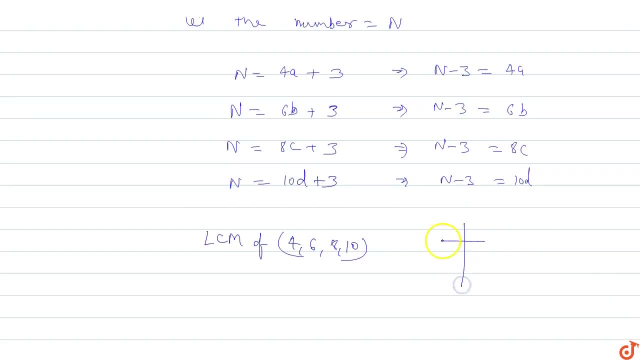 and 10.. So we will get LCM of 4,, 6,, 8 and 10.. So 2c divided by 2,, 3,, 4 and 5.. Again 2c divided by 2,, 3,, 4 and 5.. So 2c divided by 2,, 3,, 4 and 5.. Again 2c divided by 2,, 3,. 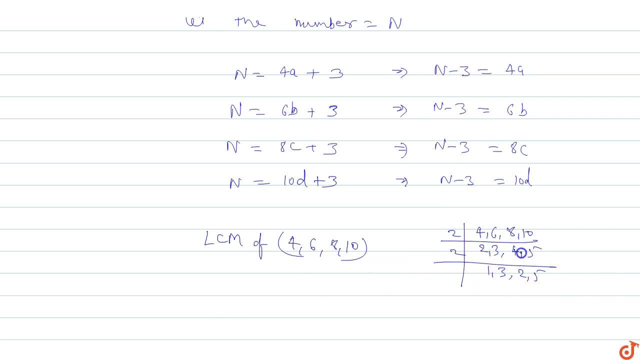 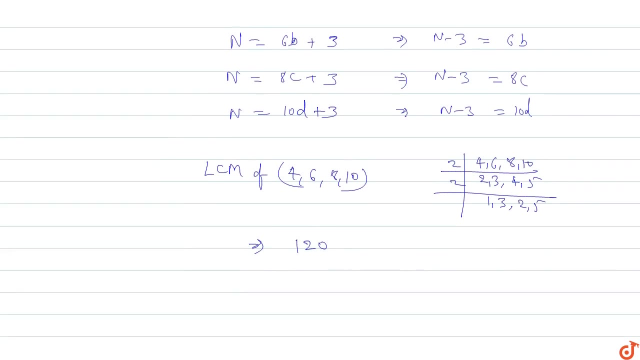 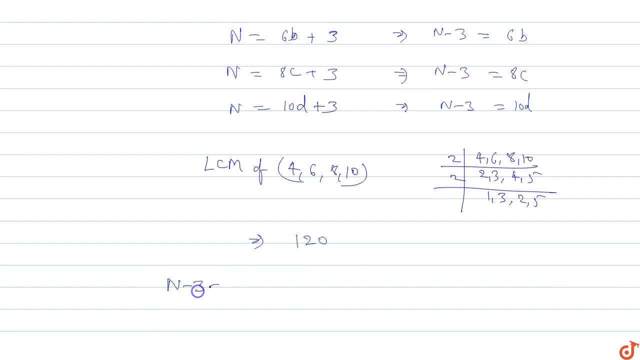 will be 1, 3, 2 and 5. so LCM of 4, 6, 8, 10. we will get LCM of 120. what will be? 120 means n minus 3 equals to 120 times of m. means n minus 3 number will be 120 times of m. so the question is smallest positive. 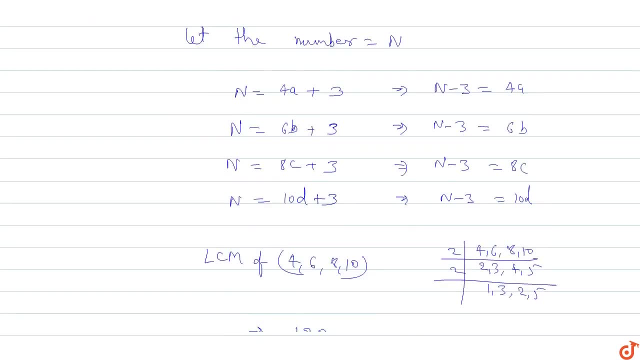 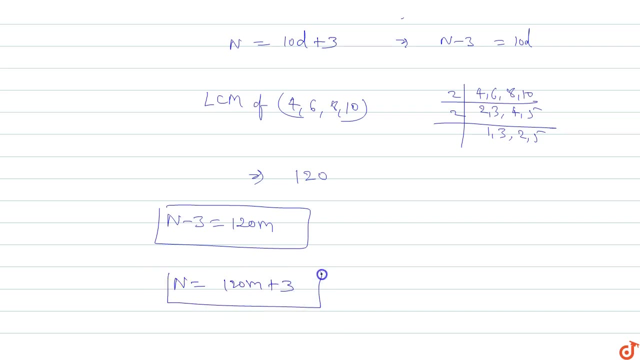 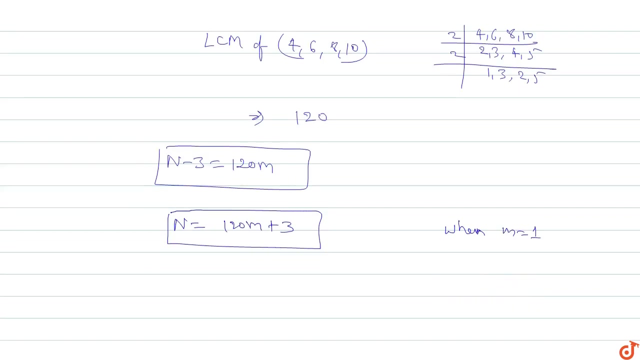 integer when divided by 4, 6, 8, 10, then remainder is 3. so smallest positive number, yeah, like 120 m plus 3, small as pose to number lover. when M equals to one, m equals to 1, so m equals to one. for well, Mary period, bar nn. 20 plus 3, so 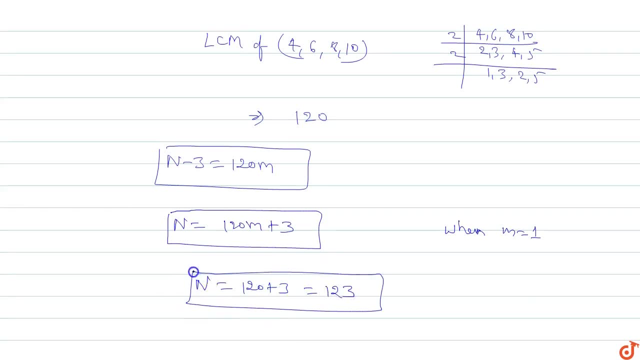 this goes to 128. the smallest positive integers when divided by 4, 6, 8, n, then, remember, is 3, so this number is smallest positive integer number is 123. okay, for more sports, positive integer 1 plus say 123 when I'm a good.